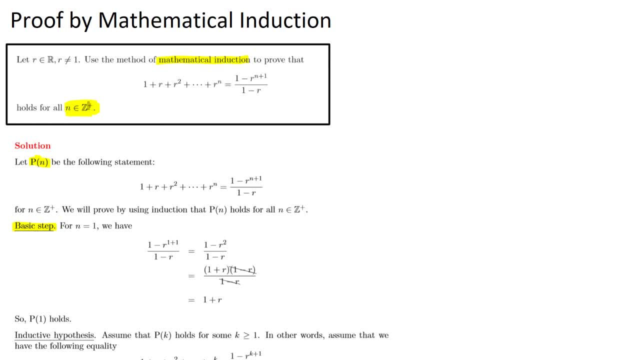 positive integers. So the first value there would be one, the first positive integer. So that's why we use n equals one for our basic step. So we just sub n is equal to one into both sides of this equation. So if we have a look at the right-hand side, if we subbed one in for n, we'd just get 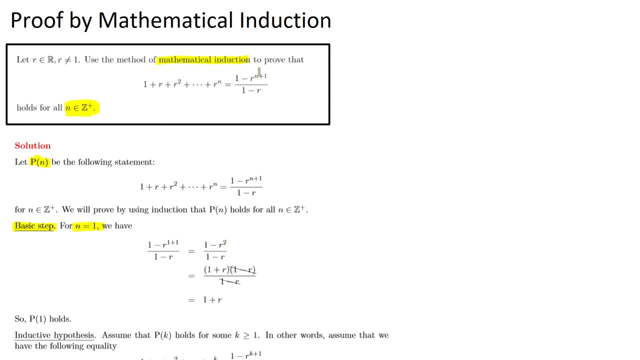 one minus r to the one plus one. so one minus r squared and we'd still have over one minus r here. And then one minus r squared is a difference of two square. This is one plus r, one minus r. You can see here the one minus rs. cancel. 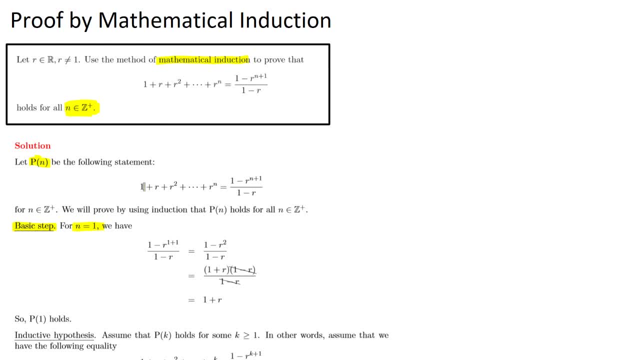 out. So we'll just have one plus r, and that is what the left-hand side would be If we had. if n was one, we'd just have one plus r to the power of one. So we have proved that the left-hand 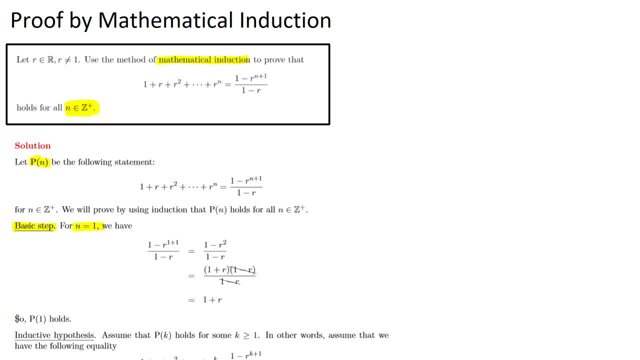 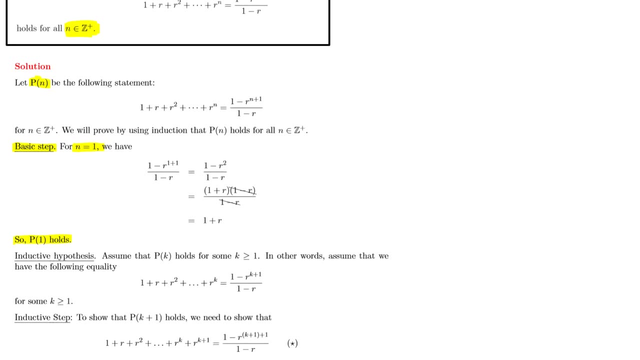 side equals the right-hand side for our basic step. So we can say so: p of one holds. Okay, that's the proof of the basic step. So if p of one holds well, does that then mean that any value of n holds? And that is what we do in the 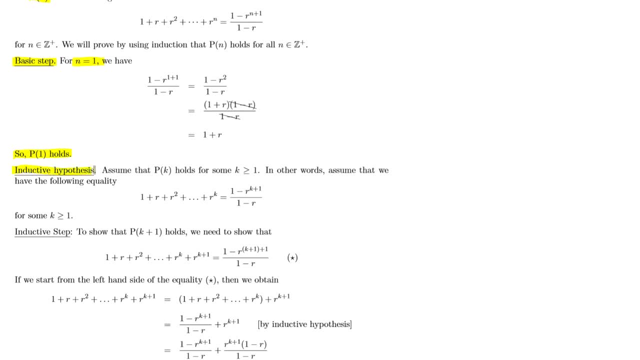 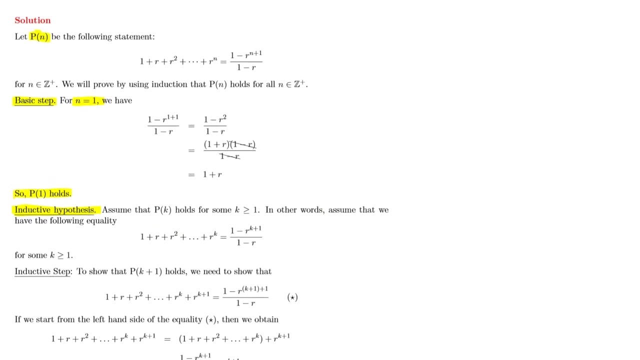 inductive hypothesis step. So the inductive hypothesis step. what this is saying is: let's assume that p of k holds for some value of k which is greater than or equal to one, And in other words, we want to assume this equation here, and it's the same equation as the one in the. 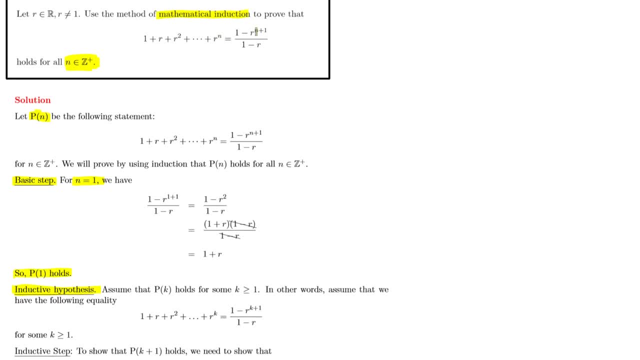 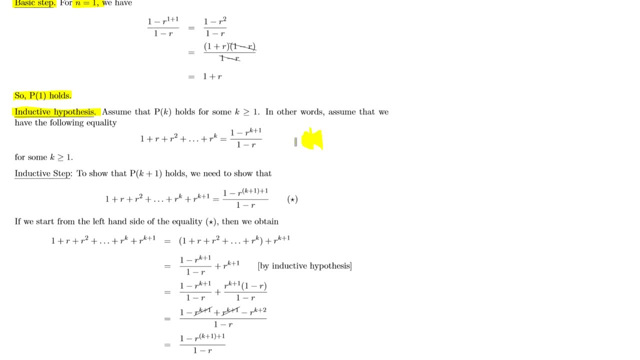 question, but we just replace n with k And we just write out that equation, which is what we've done right here Now. this is all we need to do in this step, in the inductive hypothesis step. We're going to use this equation here later on, So it is quite important that we do state it and 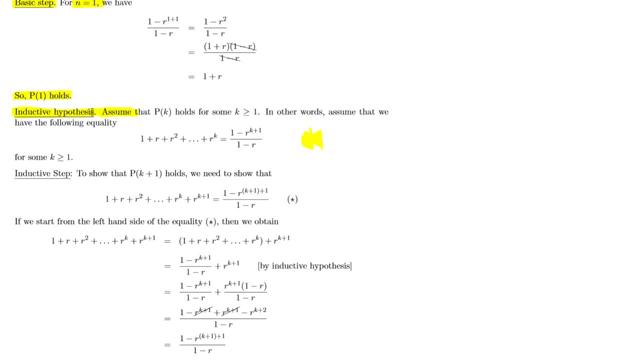 make this assumption. The assumption is very important. Okay, now we use the inductive step. This is the big step in the question which requires you to have some algebra skills And what this inductive step is: to show that p of k plus one, the next value up from k, to see if that holds. And if that holds. 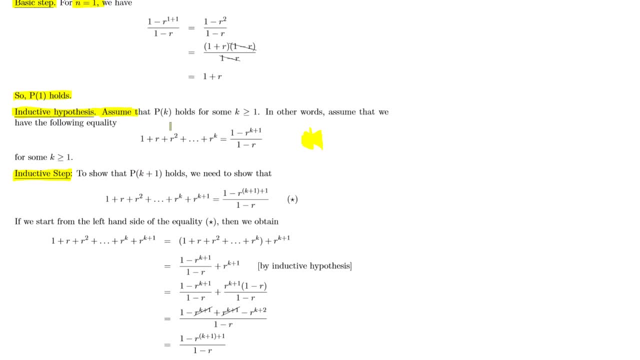 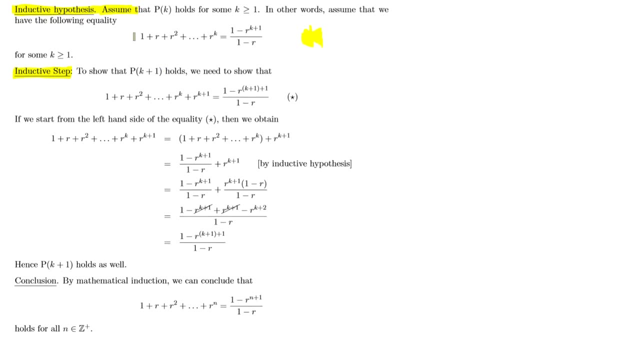 we can then draw our conclusion that the proof is a successful proof. So in this step here, what we want to do is we want to write the same equation as above as this one here, but we go to instead of k, we go to k plus one, So it's going to be one plus r. 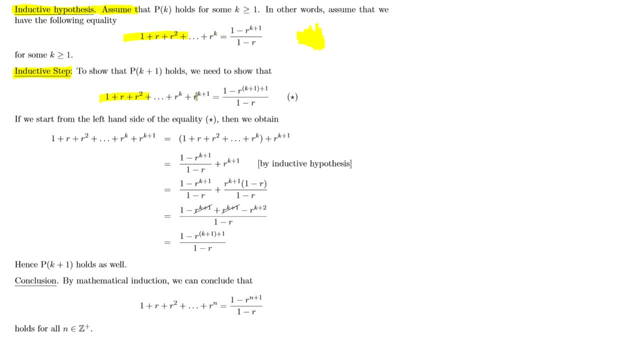 So this is the same as this, And then r to the k, and then r to the k plus one, And on the right-hand side we replace k with k plus one. That's what we have done here And this is the one we want to prove. So I put a little star next to this because 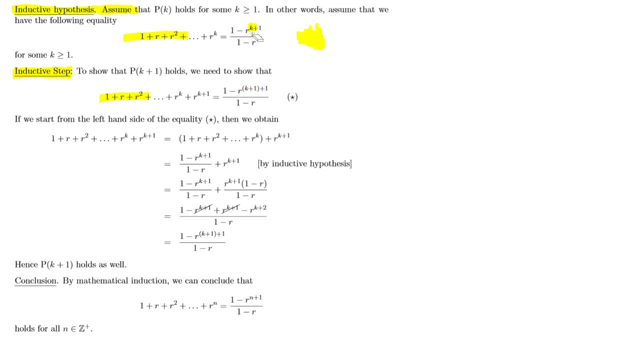 this is the key line here that we want to prove. Okay, so if we start from the left-hand side of this equation, this left-hand side, here our goal is to use algebra with this left-hand side and to finally, hopefully finally- make it equal to the right-hand side, using some assumptions. 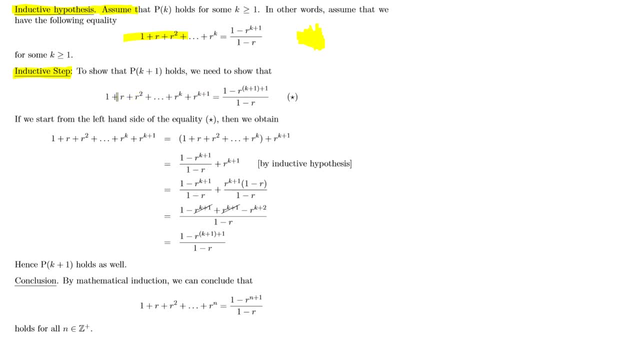 that we've made above. So what we can do here is we can realize that one plus r plus r, squared plus r to the k, this whole section here. we did have some expression for this and it's from the line up here: That's one minus r to the k plus one over one minus r. We already know that this highlighted. 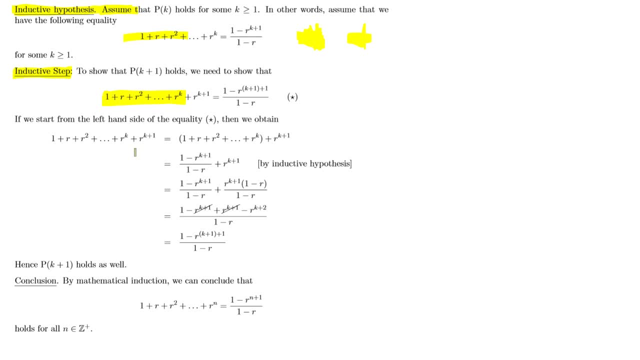 yellow bit here is equal to this. So if we work with this left-hand side, we know that this section here is just this here from the assumption line of p of k. So I've replaced it with this, and then we still have our plus r to the k, plus one That's by our inductive hypothesis. 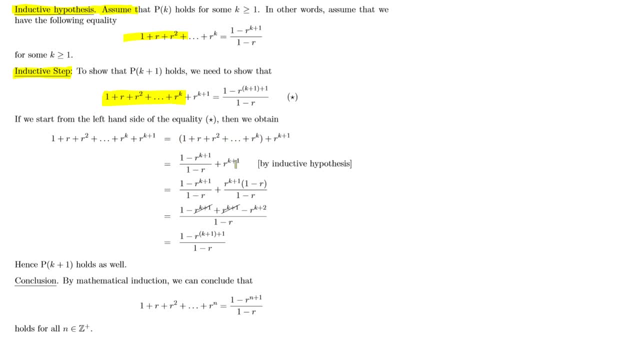 Now, from here we need to use some algebra. So with this r to the k plus one, I want to try and get this with the same denominator, the common denominator. So I'm going to multiply it top and bottom. I'm going to multiply this bottom by one minus r, which is why I have the one minus r and the one minus r. 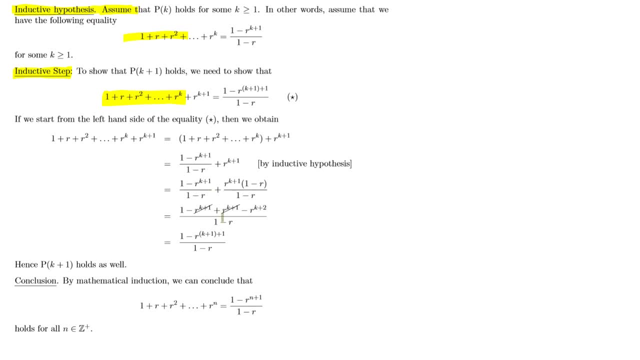 And now that we're adding the two fractions with a common denominator, we can bring them all over the same denominator, which is what we've done from this step to this step here Now, on our top lines, we're going to have one minus r to the k plus one, and then plus r to the k plus one minus r times r to the k plus one. 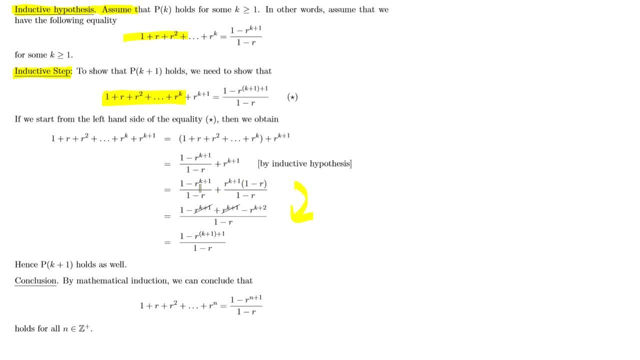 And I'll. I'll show you the algebra steps there. but you'll notice that the minus, the k plus one and the positive r to the k plus one, they cancel out. just with your indice laws here. if we have r multiplied by r to the k plus one, we know that we add the powers. 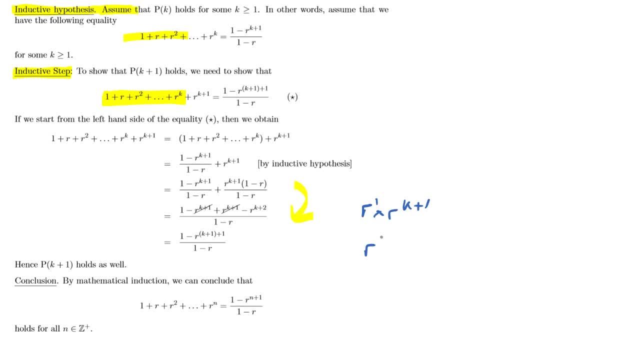 so this will become r, and then one plus k plus one, which is k plus two. so that's where this k plus two here came from. now, from here we know that k plus two is just k plus one plus one, and hopefully you, you, you stop here and you realize our answer, what we're up to here, this: 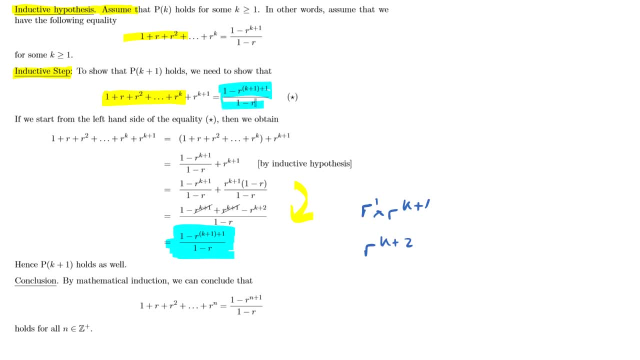 is what we wanted our answer to be in this step. it's one minus r to the k plus one plus one, all over one minus r. and once we have done that, once we have used algebra with this left hand side to get an answer which was the same as what we wanted on the right hand side, we can say: hence k of p of. 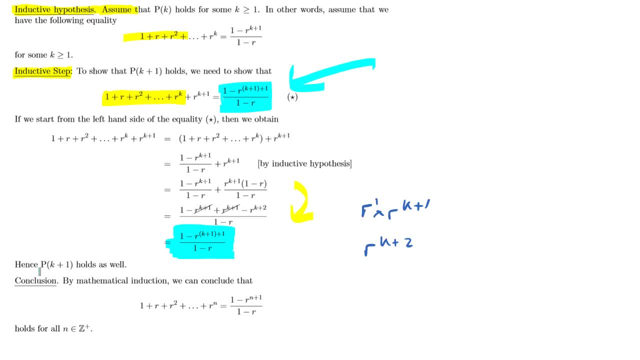 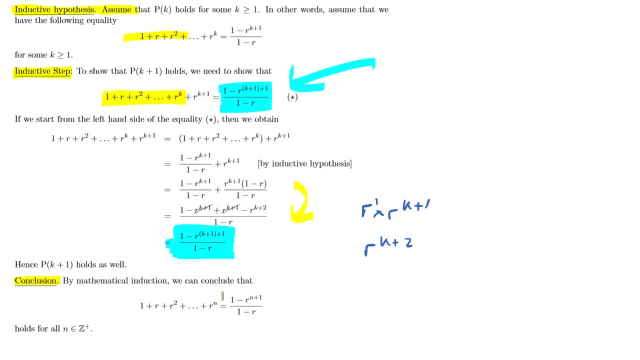 conclude that- and we have our proof here- holds for all values of n, because we know that p of one holds, and then if we made the assumption that p of k holds and p of k plus one then held, so that means, uh, it's a very important one. and then we have our proof here: holds for all values of n. 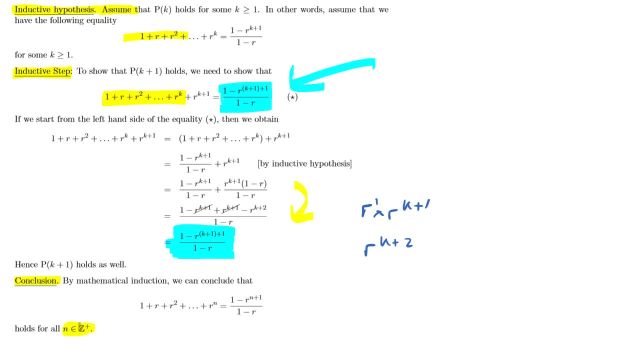 which are positive integers. okay, so well done. if you got to the end of that video, this is a. this is a classic mathematical induction question. that your question that you're doing might look a little bit different to this, but the steps are the same. you need to state your proposition, you need to have 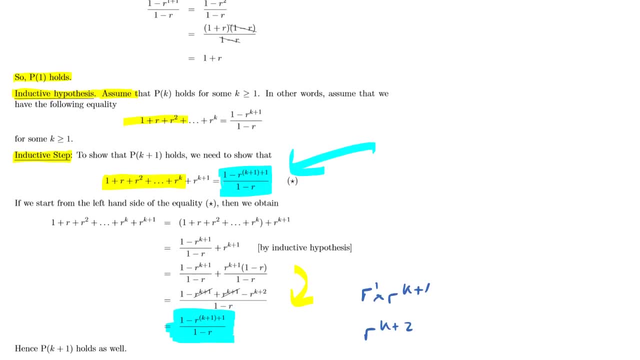 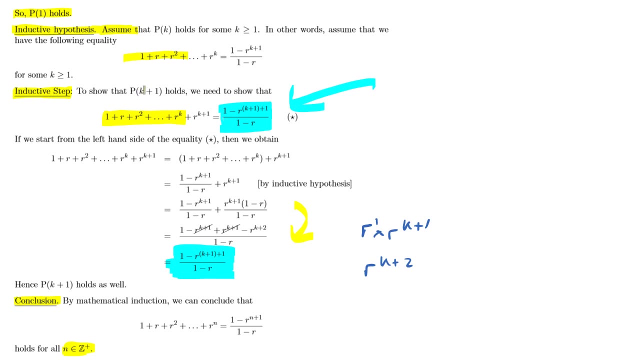 the basic step. you need to have your inductive hypothesis where you assume p of k and then you need to show that p of k plus one holds, and then up to there you need to have your inductive hypothesis where you you haven't actually done much work yet, you've just used the template. and then this is: 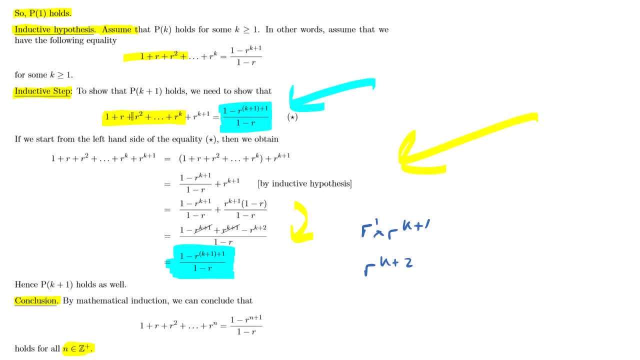 where all of the marks are. this is where you need to use algebra and you need to get this left hand side to try and equal the right hand side okay, so i think if you try maybe three or four of these questions, you should get a good feel of this topic. so good luck.